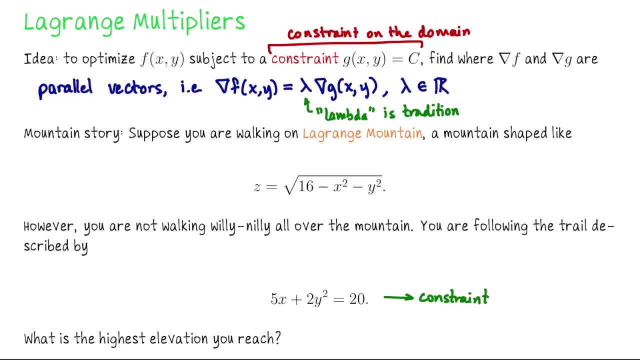 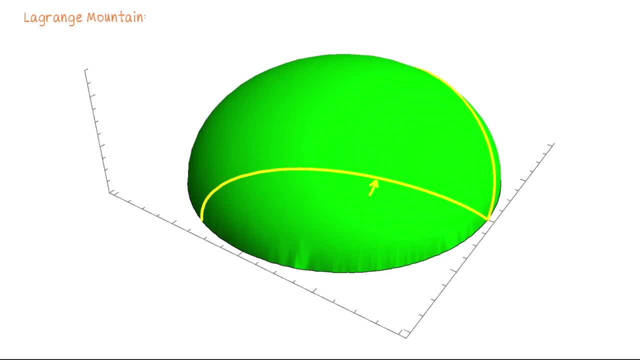 let's find my maximum height on the trail. Okay, so here's Lagrange Mountain, and I've highlighted here the trail. So it turns out there is a summit to this mountain, but I'm not a very good hiker and we're not going there. 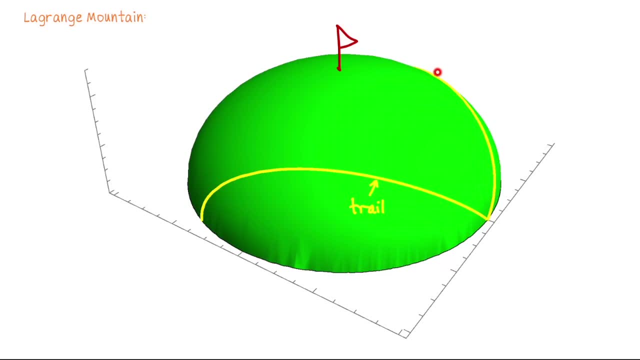 We are just going to follow this path. So this is a constraint we're putting on the x and y coordinates in the domain. You see, the domain down here is like the floor of this graph: 5 times my x coordinate plus 2 times my y coordinate. 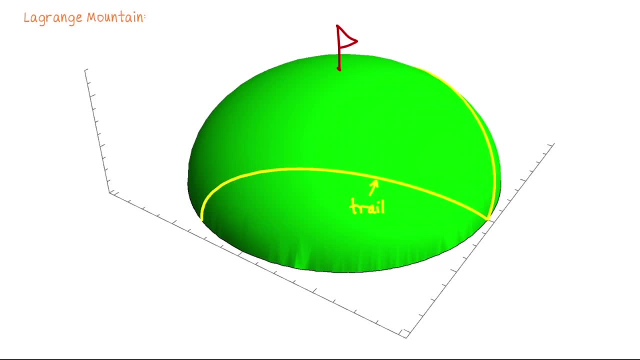 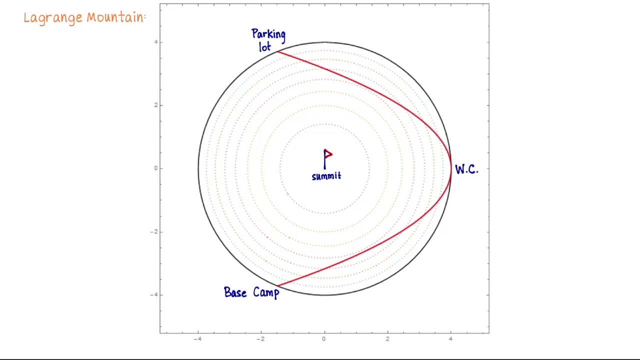 squared needs to be 20.. We are only considering points on the mountain that satisfy that property. So, given that constraint that we're stuck on this trail, it seems like the highest elevation I reach is right around here. Let's take a quick glance at the theory behind the Lagrange multipliers. So here, 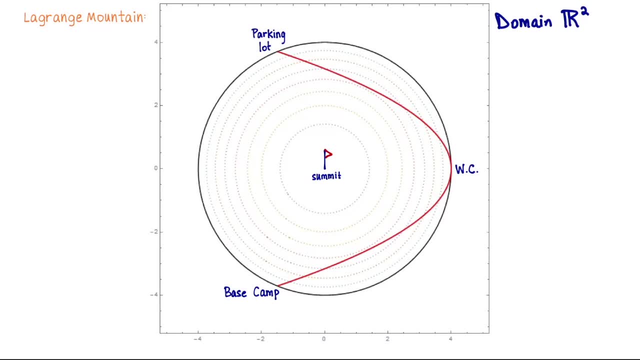 I'm looking strictly in the domain. The horizontal axis here is the x-axis and the vertical axis is the y-axis. This domain, R2, is where I'm trying to sketch a topographic map of this mountain together with my trail, So you can see both superimposed on the same. 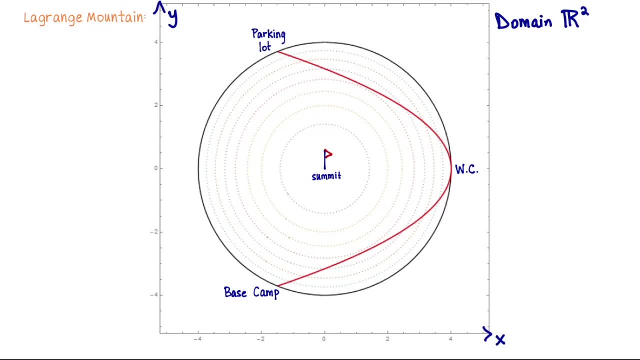 picture. What we're going to do is reinterpret this topographic map in terms of level sets of functions. The first function, f, is going to be the function for the mountain. So this is: z equals f of x, and y equals the square root of 16 minus x squared minus y squared. And then the second function: 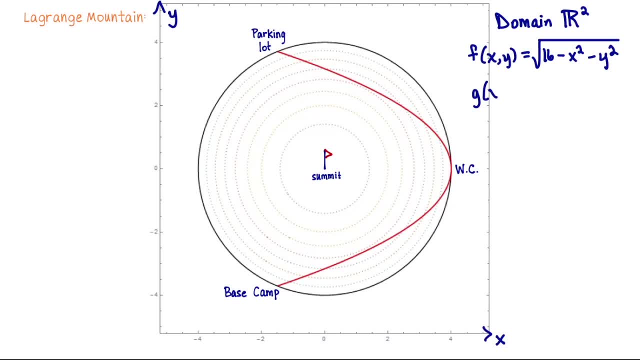 I'll create so that the path that we're following is a level curve for that function. So let's let g of x and y be 5x plus 2y squared. The domain R2 is not just the domain for f, it's also the 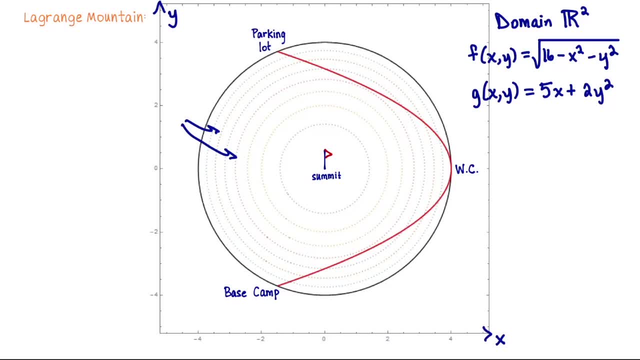 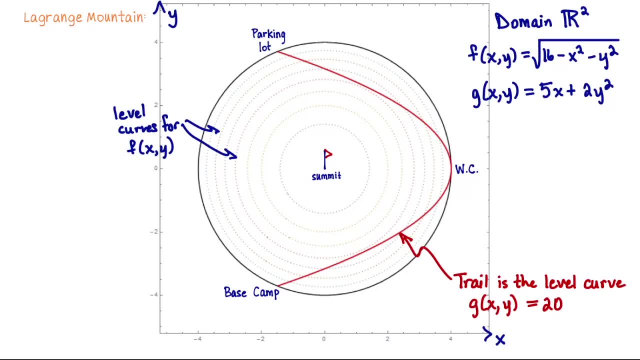 We set it up that way because our trail was following the constraint that 5x plus 2y squared equals 20.. So now I'm reinterpreting that constraint as the level curve for this new function g of x and y. We know that the gradient of a 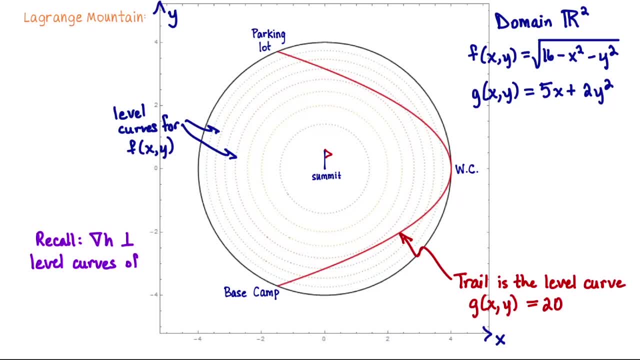 function is perpendicular to its level curves. Let's start first with the gradient of f. So if I pick any point on this topographic map and compute the gradient of f, at that point it's going to be perpendicular to the level curve containing the point. So it's. 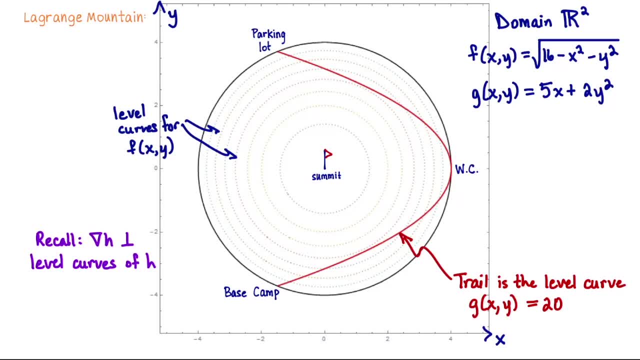 either going to point up the mountain or down the mountain, And in fact I know it's going to point up the mountain because the gradient points in the direction of increase Right. so the gradient of a function points you in the direction of greatest increase, which is going to be up towards the summit. So let 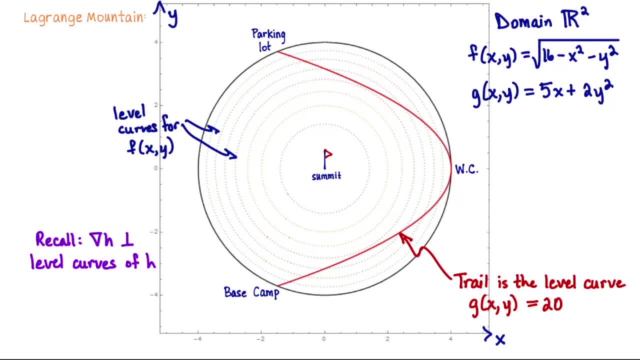 me sketch some sample gradients of f. I don't care how long they are, I'm really just interested in the sense of direction. So there's one gradient of f, Here's another gradient of f, There's a gradient of f. I sketched all five of these so that they were perpendicular to the level curve where. 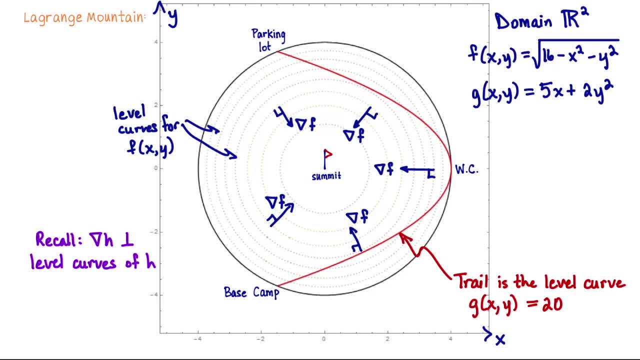 I sketched them. The trail is a level curve for g, so the gradient of g will be perpendicular to the trail. It's either pointing up or down. It's actually pointing down. You can check that by looking at the first component of the gradient. It's going to be five, So it all is going to be. 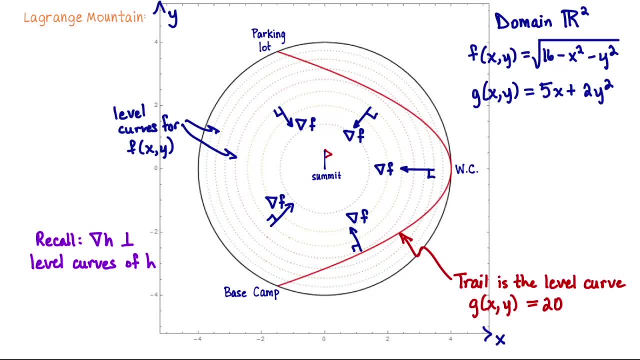 perpendicular to the level curve. The gradient of f always has to point in the direction of positive x. So there's a sample. gradient of g. It has to be perpendicular to the trail. Here's another one. Okay, so that's how the gradient of g relates to the trail. 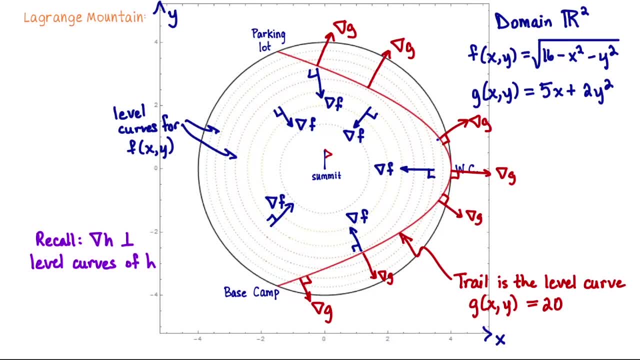 Let me draw a couple more gradients for f Now. if we follow the trail, the highest point of the gradient of g is always the highest point of the gradient of g. The highest point of the gradient of g is always the highest point of the gradient of f. 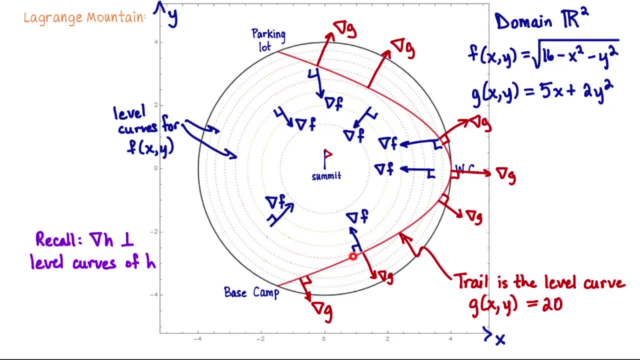 So let's start with f. So this is the highest point of the gradient of g, And what happens here is that the gradient of f generally doesn't even have much of a perspective. What happens here is that the gradient of f is held in the upper left part of the graph. 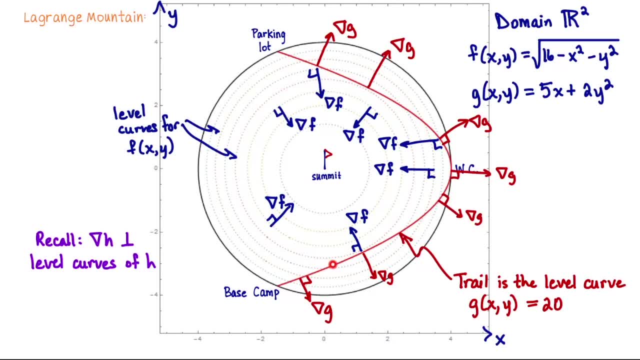 and is used to follow the top of the graph, And we want to know how it brake. The gradient of f is held in the upper left place, in the top left corner of the graph, So that's what we call the gradient of f. 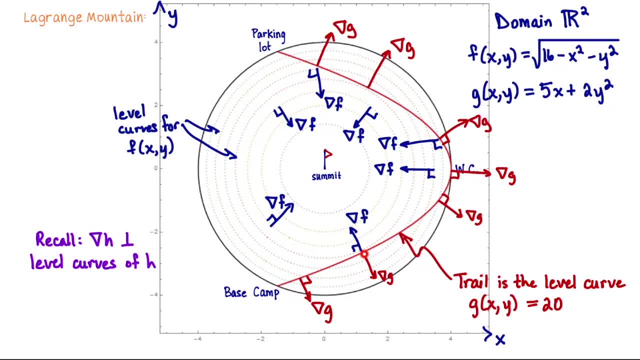 And it's held in its center. We want the gradient of f to be perpendicular to the area of the graph and we want to know how it goes. So the gradient occurs right around here And that's where our trail stops going up the elevations curves for f and starts going. 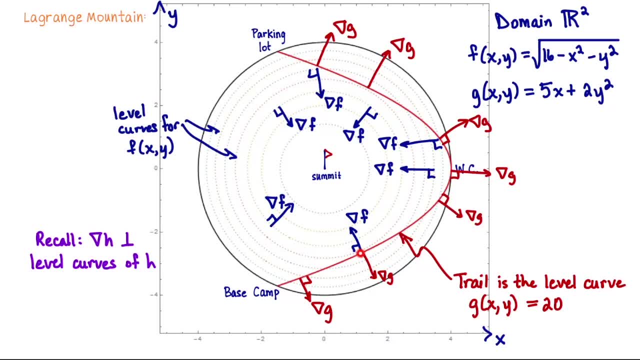 down to one of these concentric circles. Consequently, the two gradients are parallel. If you compare that to say over here or over here, you see that in general the two gradients are not parallel. So this was just an illustration of the general principle. 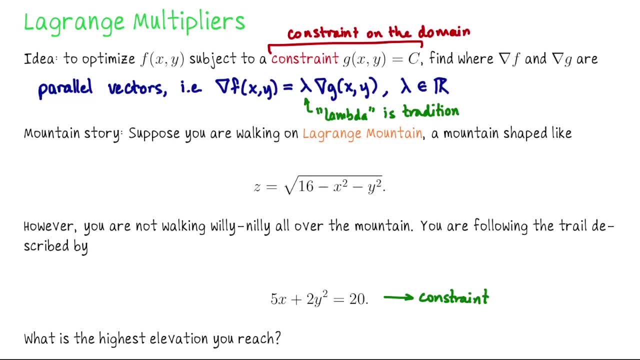 which is that if you want to optimize f, it's the height we reach on this mountain. subject to a constraint: my trail. you want to compute their gradients and figure out where they're parallel. In other words, one can be written as a multiple of the other. 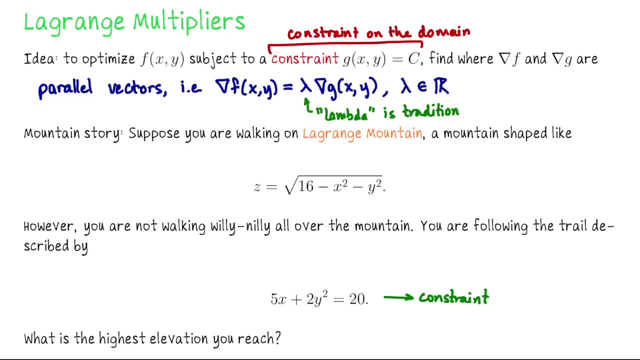 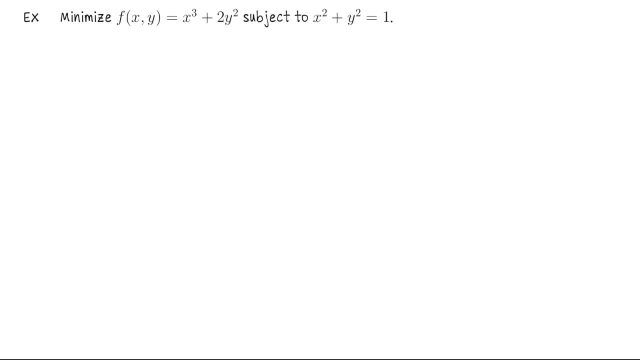 It doesn't have to be positive or negative. They could point in the same direction or opposite directions, They just need to be parallel. Okay, let's do one example. We are going to minimize the function f of x and y equals x cubed plus 2y squared. 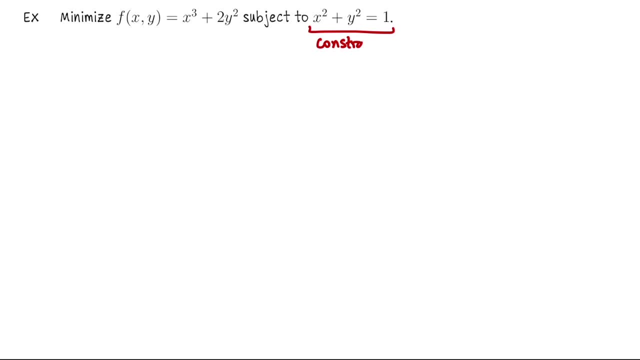 subject to the constraint that x squared plus y squared equals 1.. Okay, let's do one example. We are going to minimize the function f of x and y equals x cubed plus 2y squared, subject to the constraint that x squared plus y squared equals 1.. 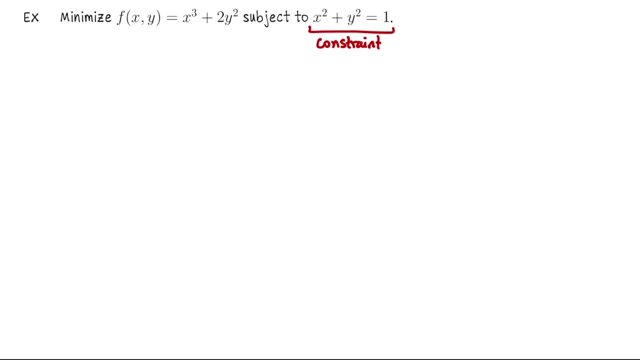 Okay, let's do one example. We are going to minimize the function f of x and y equals 1.. In other words, I'm not looking to minimize this function in general, I'm only looking to minimize it over the unit circle. 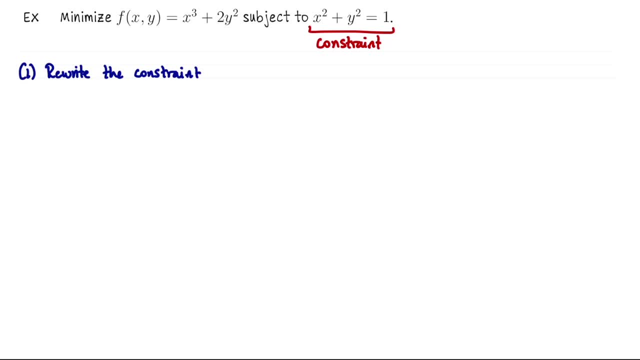 In general, the first step to these problems is, if necessary, to rewrite the constraint as the level set of some new function, g. So let's let g of x and y equal, x squared plus y squared. Then our constraint is that we need to live on the level set. 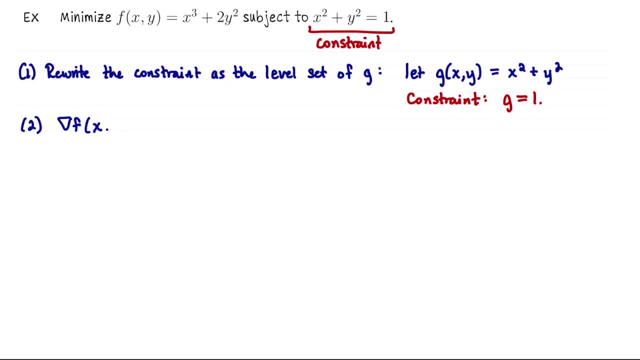 g equals 1.. The second step is to compute the gradient of f and the gradient of g. The third step is to set up a system of equations that x and y would need to satisfy together with the multiple lambda, in order to have the gradient of f equal to lambda times the gradient of g. 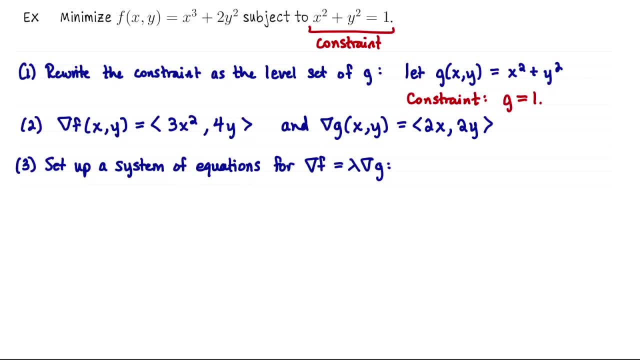 Okay, if the gradient of f equals lambda times the gradient of g, then that means the first coordinate of f is lambda times the gradient of g, Then that means the first coordinate of f is lambda times the first coordinate of g. So for the x coordinates I can say that 3x squared equals lambda times 2x. 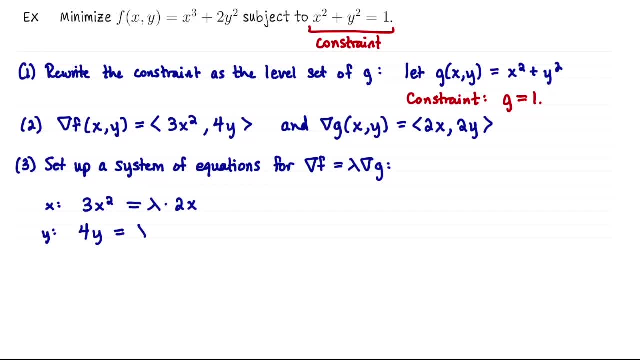 For the y coordinates I can say: 4y equals lambda times 2y And that's it for the coordinates. But if you look at this, this is two equations for three unknowns. We don't know x, y or lambda. 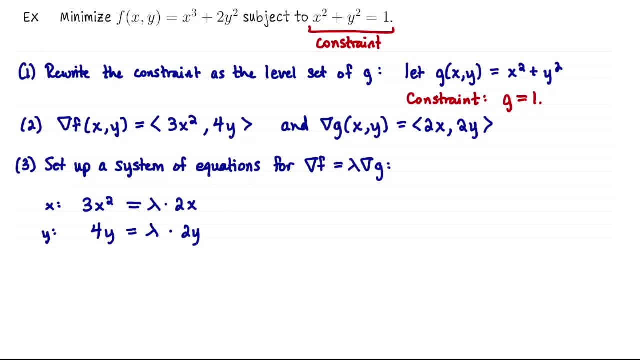 So there's always a final equation that you amend into this system, and that is the equation given to you by the constraint. We need x squared plus y squared to be 1.. So that's our system of equations. Now, the system that results from this process can be easy to solve. 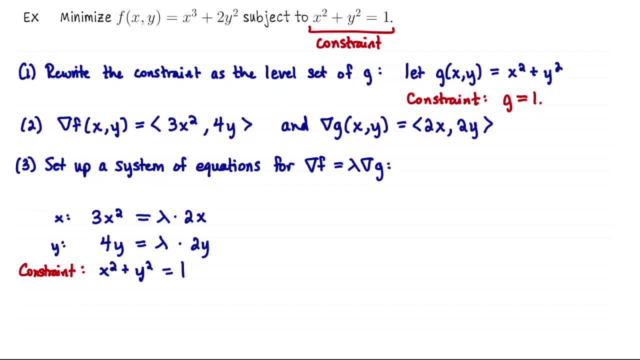 It can be very hard or impossible to solve by hand. It really depends on the functions you're given. So, systematically, here's what I do: I try to determine the conditions that would make each equation true. So the first equation would automatically be true if x equals 0.. 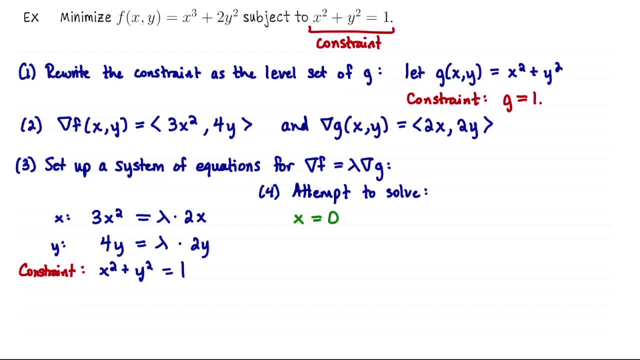 If x isn't equal to 0, then I can divide both sides by x, and I get 3x equals 2 lambda. The second equation is automatically true if y equals 0. If not, I can divide both sides by y- actually by 2y- and I get lambda equals 2.. 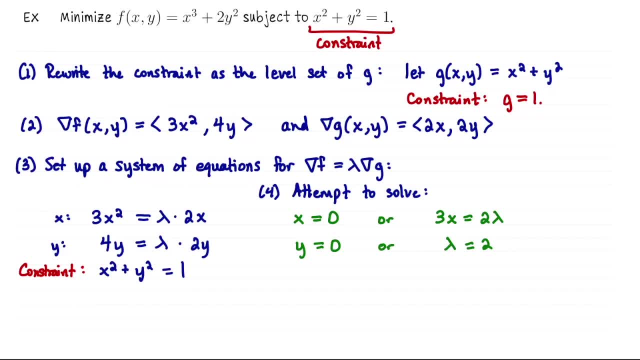 Okay, now I just play. choose your own adventure. So let's suppose x equals 0.. If x equals 0, can I let y also be 0 for the second line? And the answer is no, because that would violate the constraint. 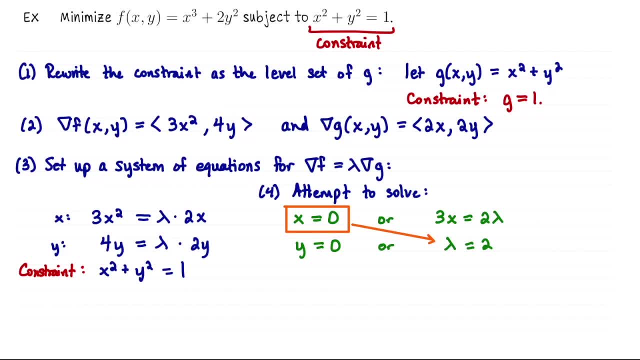 So x equals 0 can only be paired with the possibility that lambda equals 2.. Okay, so if x equals 0 for the first equation, it must be the case that lambda equals 2 for the second equation. I don't have anything yet for y, but just go down to the constraint. 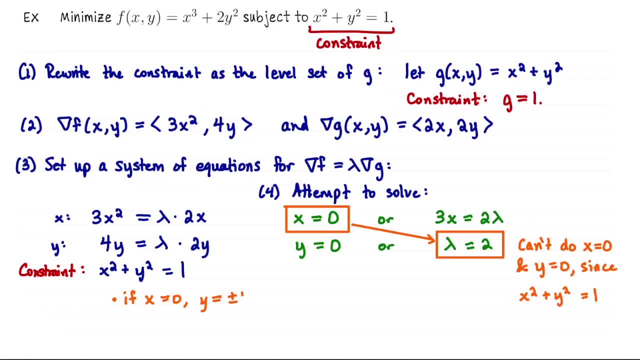 If x equals 0, y is plus or minus 1.. If we're looking to minimize this function, we would then check 0, 1, and 0, negative 1, and we would ignore the fact that lambda equals 2.. 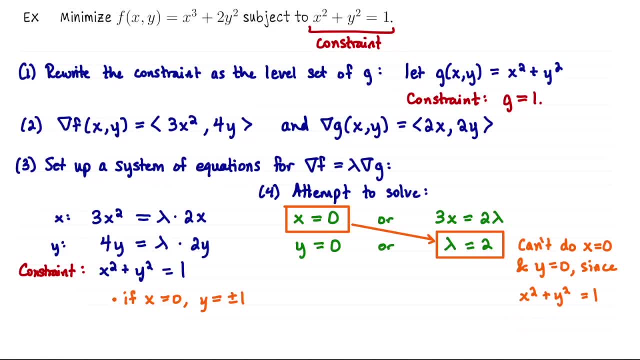 We would have found the points. Lambda doesn't necessarily have to come true. It doesn't necessarily have to come into your calculations in the end. Okay, that's it for x equals 0.. So if it's not the case that x equals 0 for the first equation, it must be the case that. 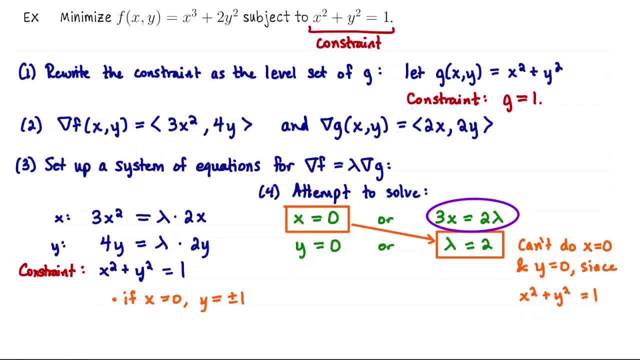 3x equals 2 lambda. So if 3x equals 2 lambda, can y be 0?? And the answer is sure: why not? If y equals 0, x is plus or minus 1. And we don't need anything to do with lambda. 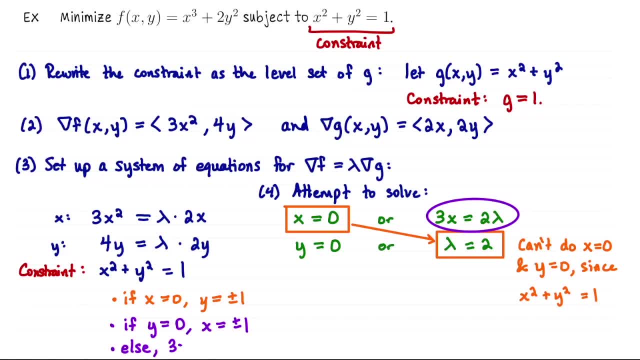 If it's not the case that y equals 0, then 3x equals 2, lambda and lambda equals 2.. So this is the only calculation where I'm using something about lambda. If 3x equals 2 lambda and lambda is 2, then 3x equals 4, which means that x is 4 thirds. 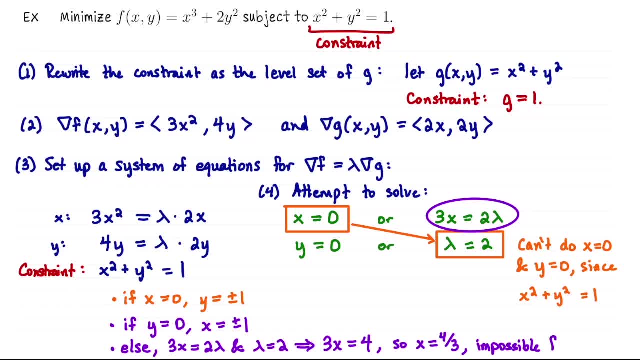 which is impossible Because that can't satisfy the equation: x squared plus y squared equals 1.. If x is 4 thirds, we can't plug it into that equation. Now I'm done with this system of equations. I considered the first possibility, that x equals 0, found the possible points associated. 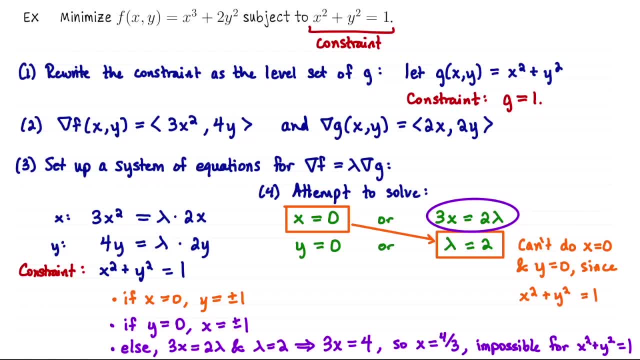 with that 0, plus and minus 1.. Considered the second possibility, that 3x equals 2 lambda, and found all the points associated with that, which is plus minus 1, 0. So we have four points to test in this function. 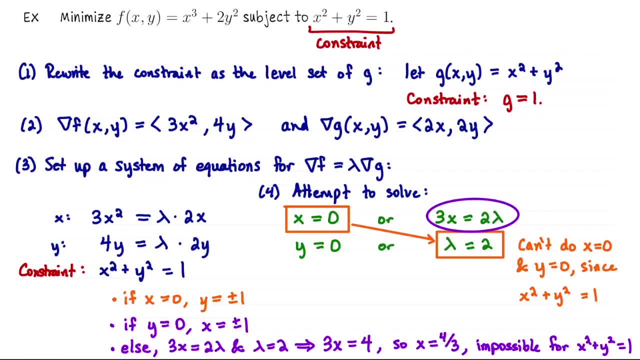 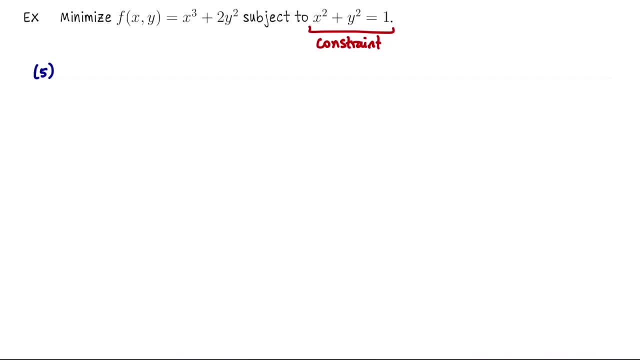 The maximum value we get will be the maximum of f sub lambda. Subject to this constraint, the minimum value we get will be the minimum. Okay, so the final step is to plug the points that we've identified into the function f of 0,. 1 is 2.. 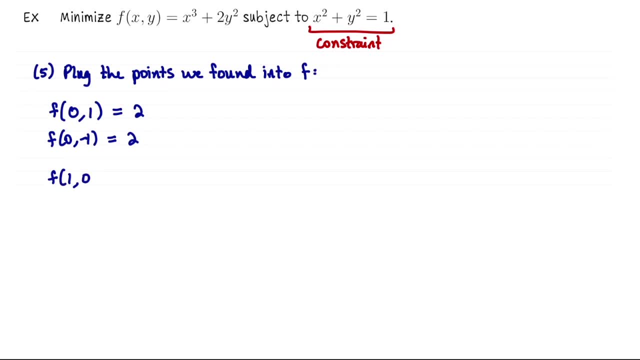 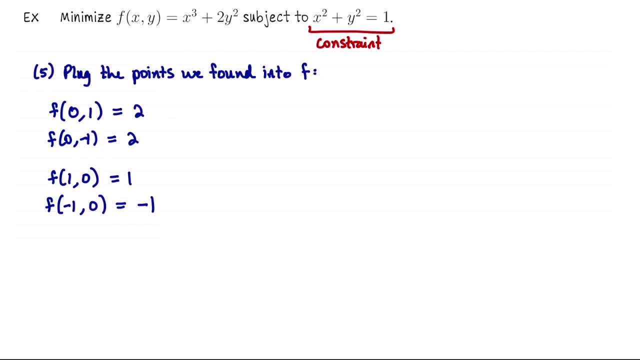 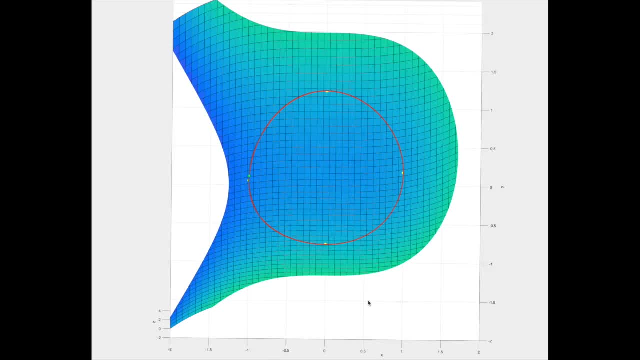 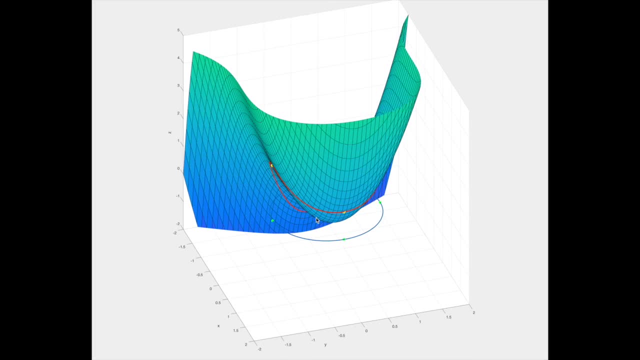 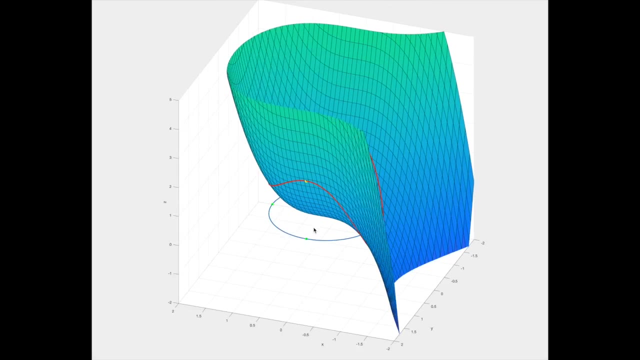 Here's a picture of this situation. So I've plotted f in general, highlighted the constraint And then plotted the constraint on f. So here you can see: on the y-intercepts, f attains the maximum value of 2.. And over at negative 1, 0, it attains its minimum value of negative 1, subject of course to 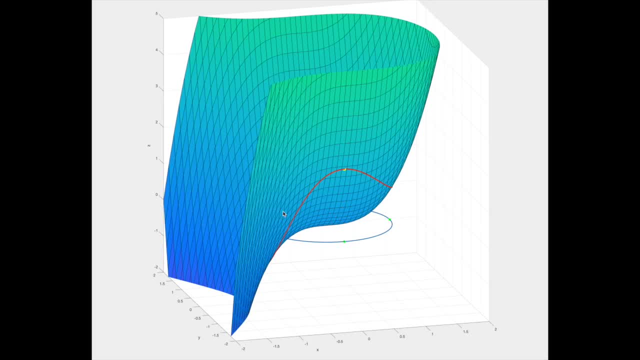 this constraint that our x and y coordinates are coming from the unit circle. That concludes our discussion of Lagrange multipliers.